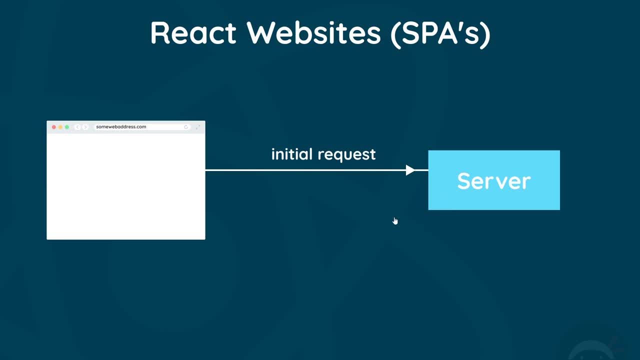 request in the browser. The server then responds to that by sending back the HTML page to the browser, But it also sends back our compiled React JavaScript files, which controls our React application. So from this point on, React and the React router can take full control. 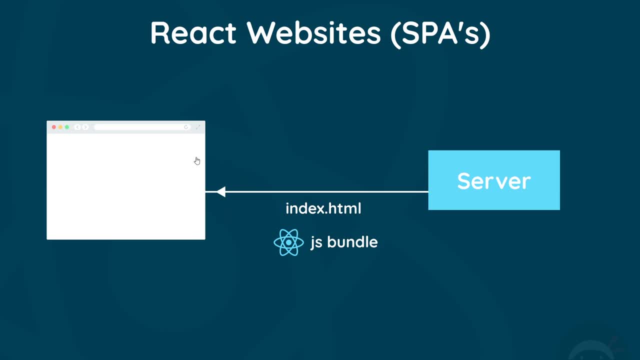 of the application. So initially, the HTML page that we get back is virtually empty, And then React injects the content dynamically using the components that we create. If we then decide to click on a link to a new page, the React router is going to step in and 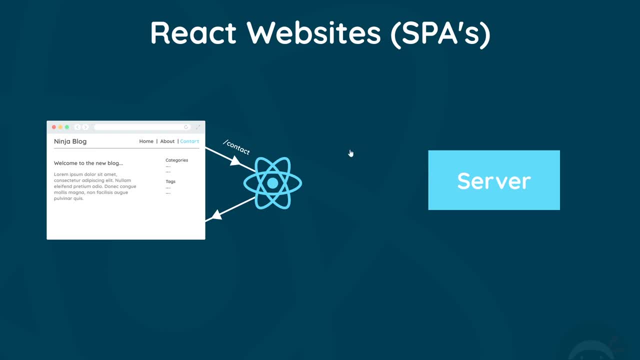 intercept that request to stop it from going to the server And instead it's going to look at the new page request and inject the required content on the screen. For example, clicking on a contact link, the React router will tell React to inject the contact. 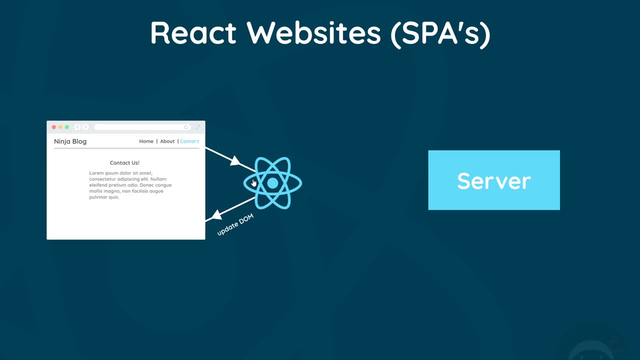 component into the browser And if we were to click on an about link, that part would always end up getting passedware. So if we wanted to have all of those all within one website, we would need our contact link in our account If we were to show a link here which would accept it from the server. 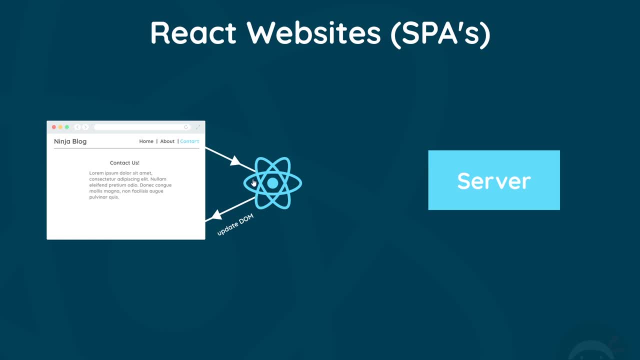 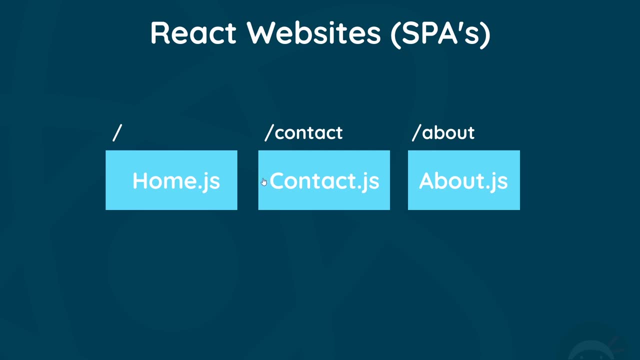 It would tell react to inject the about component and so forth. So this is generally the way the react router works. We assign a top-level component for each route or page and that component is dynamically injected Into the browser when we visit that route. Now this whole process means that we're making less requests to the server and the whole website therefore feels faster and slicker. 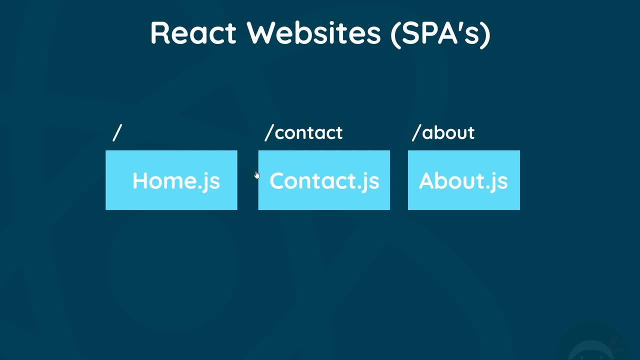 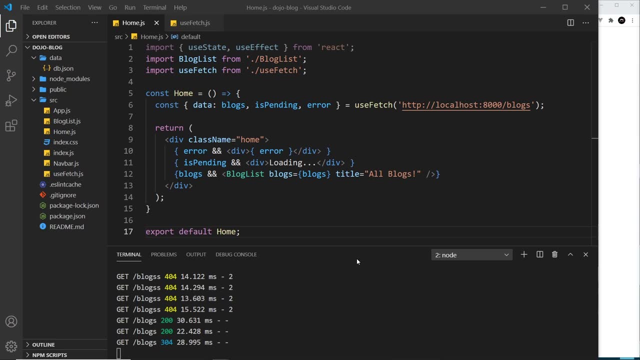 So now we know from a bird's-eye perspective how this works. Let's see how to set it up in our code. So the first thing we need to do is install the react router package, because it's not a part of the core react library. Now, to do this, we need NPM and we need a new terminal. So click on this and then we're going to type NPM. 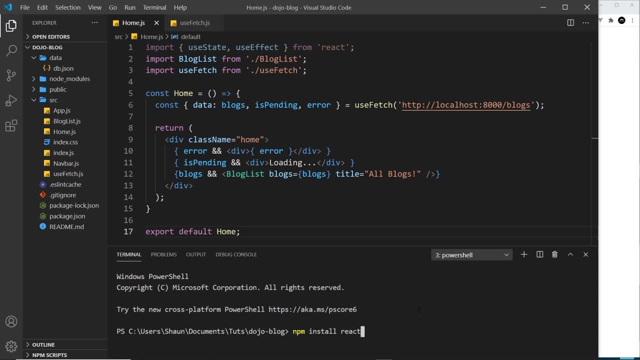 Install and then it's react, hyphen router, Hyphen Dom, and then I'm going to use a specific version and that version is five and to do that, I'm Going to say at five. now, this version is currently stable. Version six is in beta, but that might change over the coming weeks and months. 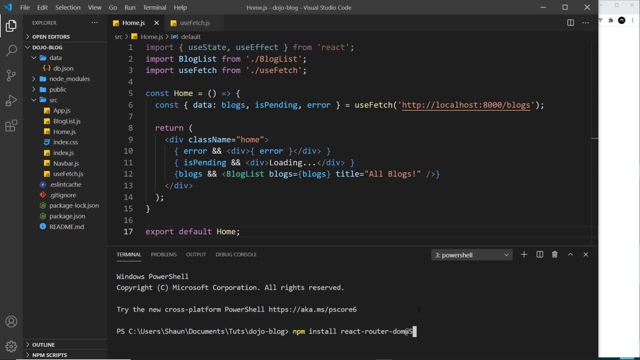 So I didn't want to use that version in this series in case it does change. But I will be doing a react router six tutorial once a stable release is here, or at least once we have a release candidate. But to follow along with this, use version five like me, and then you can always upgrade to version six in the future. 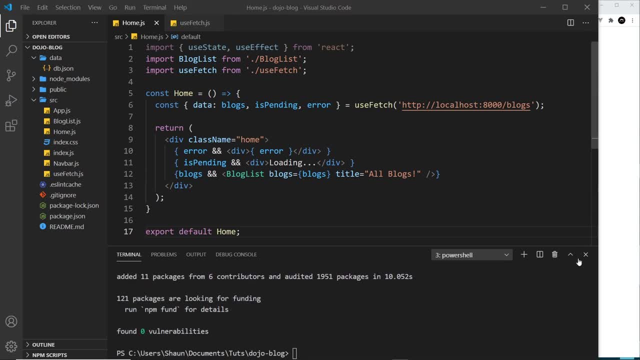 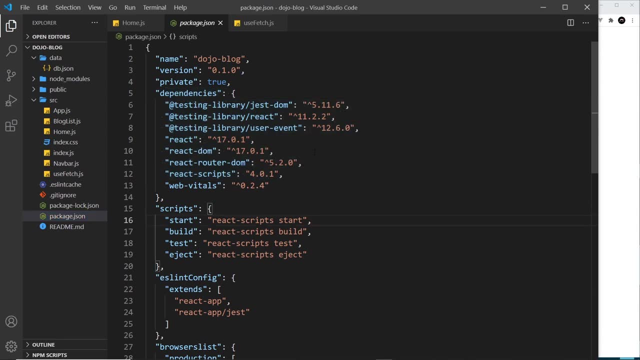 So press enter to install This and then, once that's installed, we can close this and just go to your package dot JSON file and you should see now the react router Dom package right here. So version five, point two. All right then. so remember, when we install something it goes inside the node modules folder. 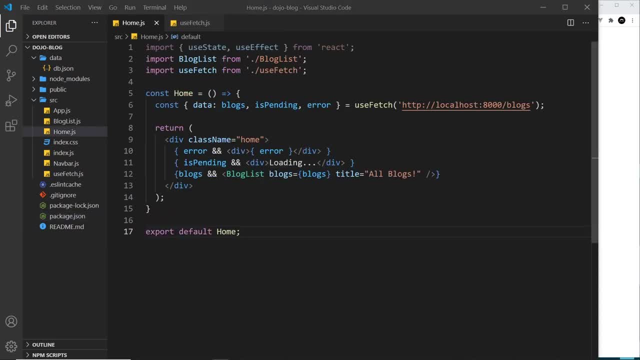 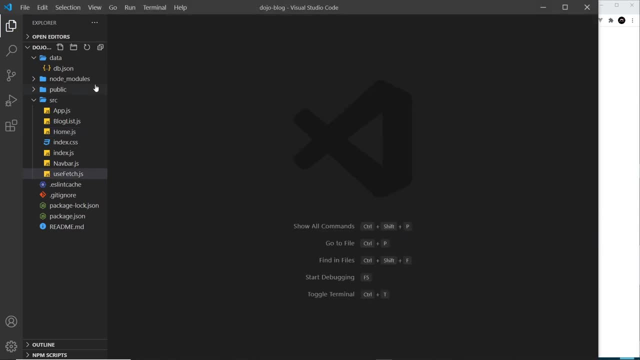 So if you're wondering where it's put that, it's inside here. So now we've installed that package, How do we actually use it and set up routing for our application? Well, the first thing to do is to go to the roots component, Which is this app dot JS file, and we need to import a few things from the react router package right here. 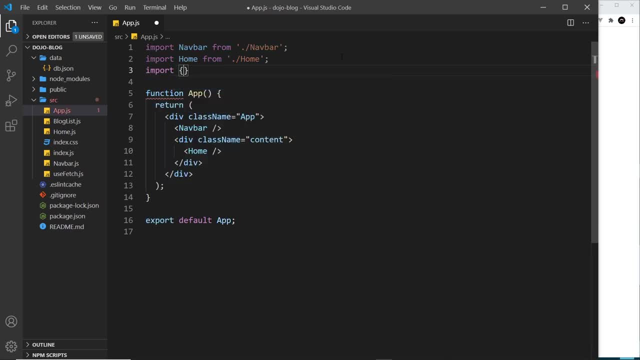 So let's do that. first I'm going to import and then we're going to destructure a few things. The first thing we need is the browser router and we're going to say as Router, and that means we can use the browser router that we're importing using this name inside this file. 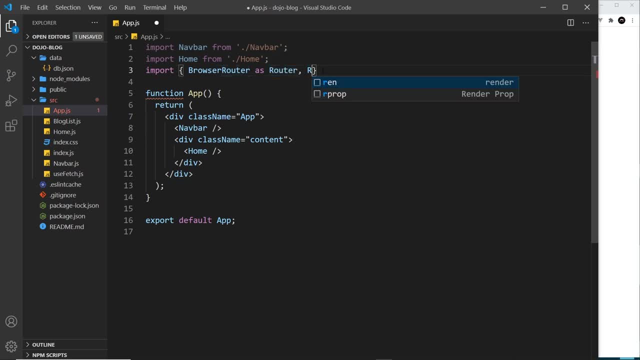 so that's the first thing we want to import, and we also want to import something called the routes components and also the switch Components. so we'll see what these do as we go forward, But for now, let's say, from react hyphen router. 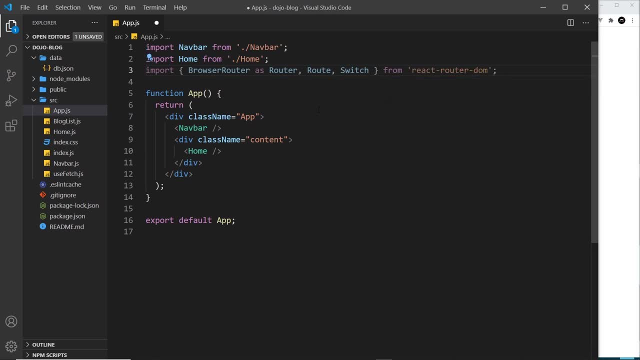 Hyphen: Dom. Okay, So now we need to surround our entire application with the router component, And what that means is that we can use the router in the entire application. all Components that are nested inside this app component have access to the router, So let us now do that. 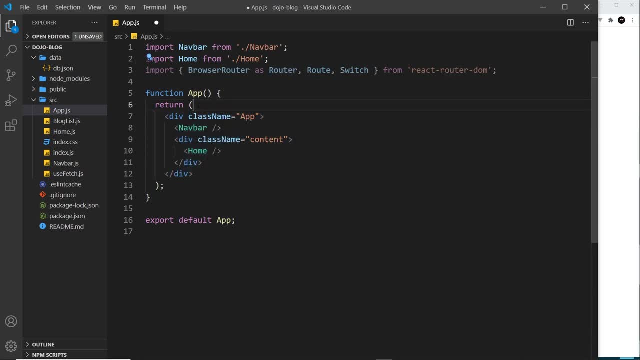 I'm going to surround this div with this router component, so router like so. and then we get the closing tag here. let's place that at the end and Scoot this in, All right. so that's the first step. The next step is to decide where we want our page content to go when we go to different pages. 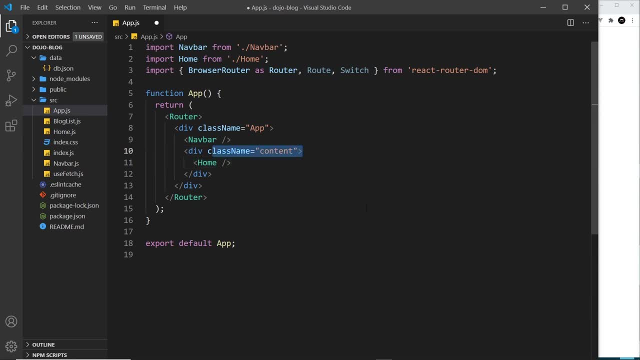 Well, I want it to go inside this div right here with the class of content. So I'm going to delete that home component right here and I'm going to replace it with the switch component, like so: Now, this switch component makes sure that only one route shows at any one time. now, 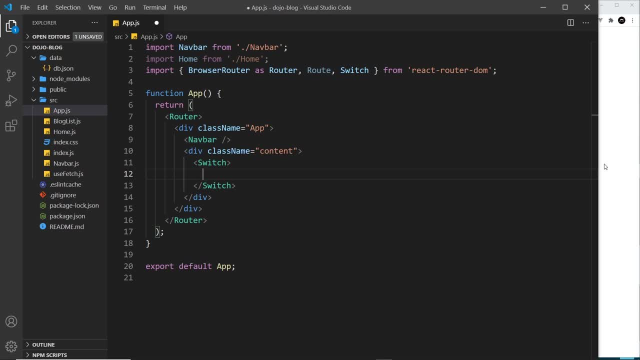 We're going to talk a little bit more later about how that works, But just know for now, all of our routes go inside this switch component. Okay, so now we need to set up our individual routes. So what we do is we create a route for each page that we have using this route component, right here now. 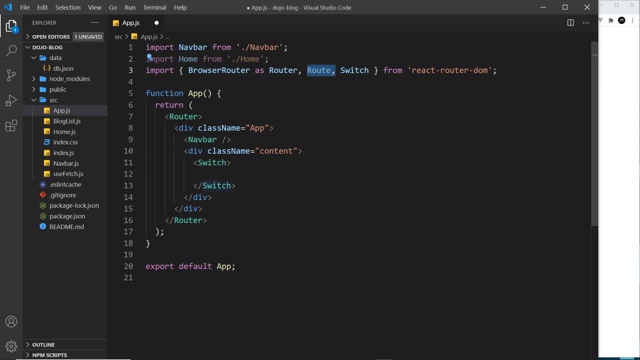 We only have one page for now, So we're just going to place one route inside This switch component, but later on we're going to have other pages and more routes inside here as well. So let's do our route for the home page, So the route component, like so, and 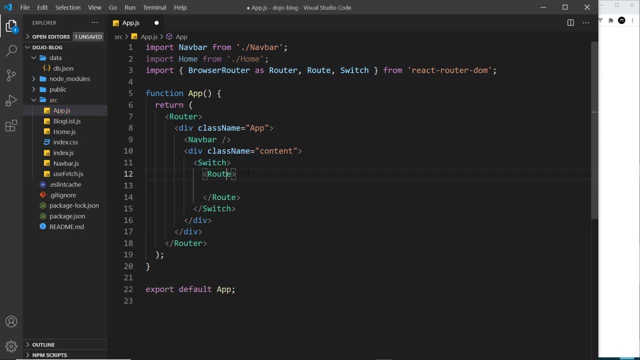 then let's get the closing tag as well, and then we need to add on a property to the route component, which is going to Be the path. now the path property. Oops, that needs to be inside the route component. Let's cut it and paste it right here. The path is basically the route. 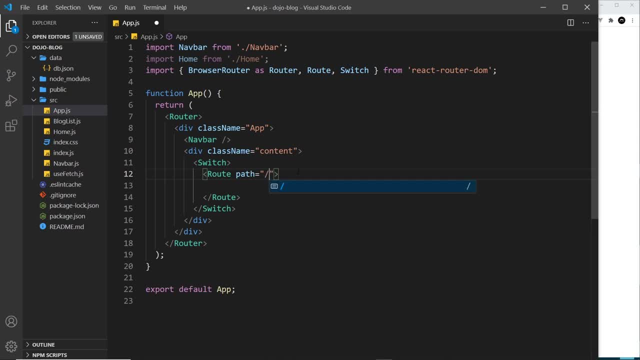 so for the home page page, it would just be forward slash right. if we were doing an about page, it could be forward slash about. if it was a contact page, it could be forward slash contact. basically, this is the path after the root of our website. so if our website was called thenetninjacom orcouk, it would be the path. 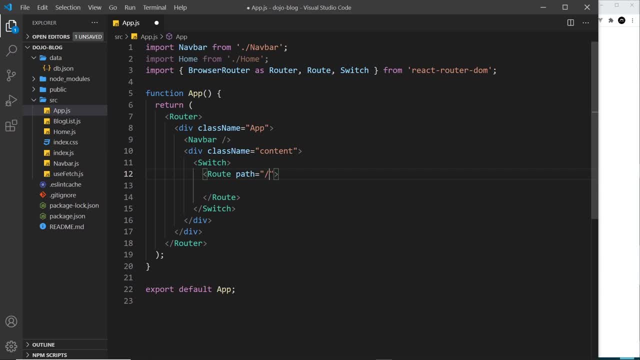 after that part of the url. okay, so this is the path for the home page, and what we need to do is nest the component inside this route that we want to show when a user visits this route. so i want to show the home component. so home, like so. and now what we're seeing is okay. 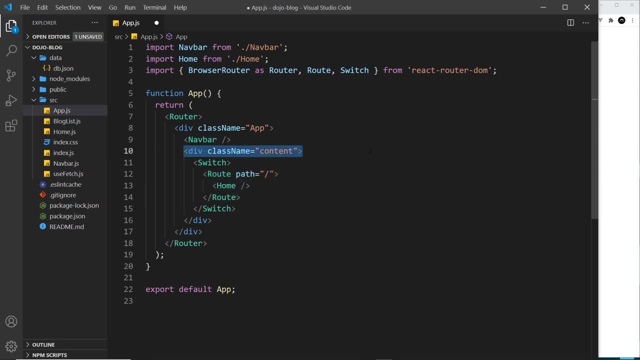 i want you to show the home component right here inside the content div when we visit just forward slash. now notice the navbar is always going to show because it's not inside this switch statement. this is here for every single route, it doesn't matter what it is.